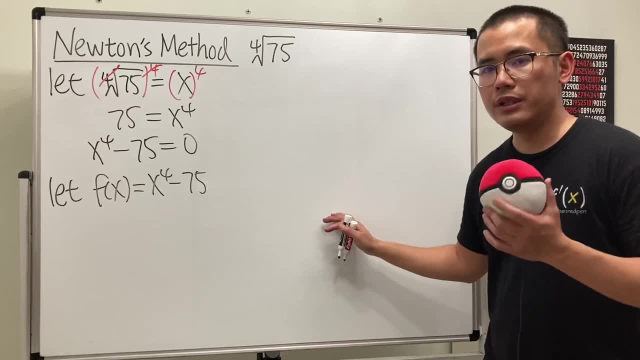 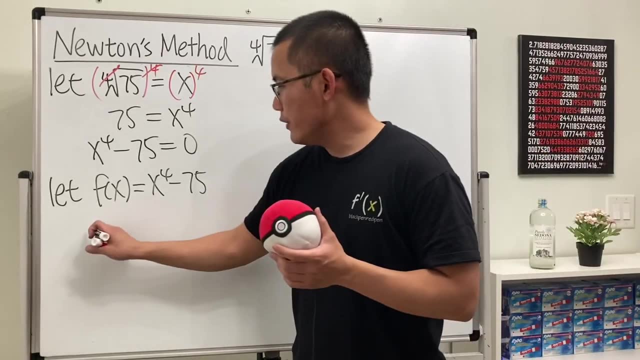 And the next thing that we need is we need to have a good initial guess. How can we do it, though? Well, let's just kind of approximate this a little bit. You see, if we have f of, let's say, 2.. 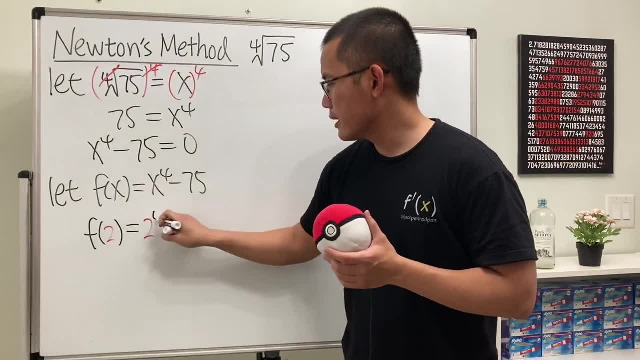 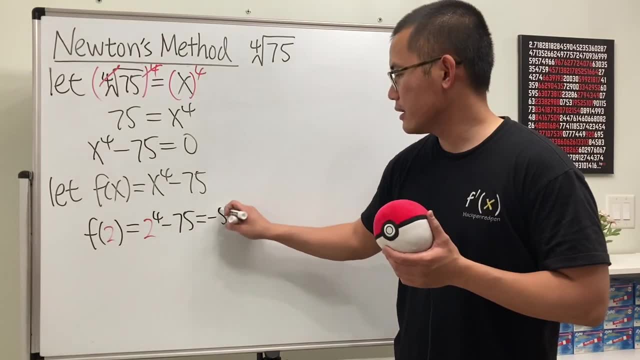 2 to the force power is 16.. Keep that in mind. And then minus 75.. Minus 75. 16. Minus 75 is negative 59.. Yeah, Okay, it's too far below zero. Okay, keep that in mind. 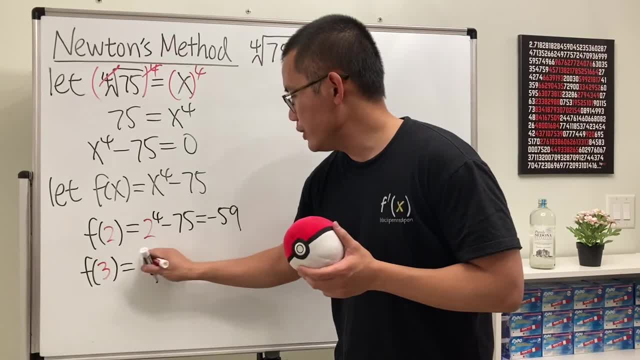 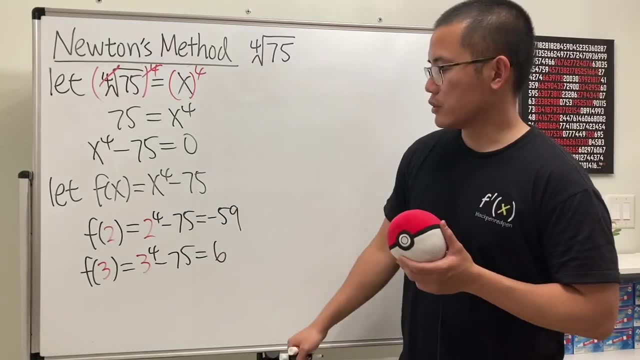 But like, if we have f of 3.. 3 to the force, power is 81. And then minus 75. And that will give us 6.. So, as you can see, we can expect that this value is going to be closer to 3 rather than 2.. 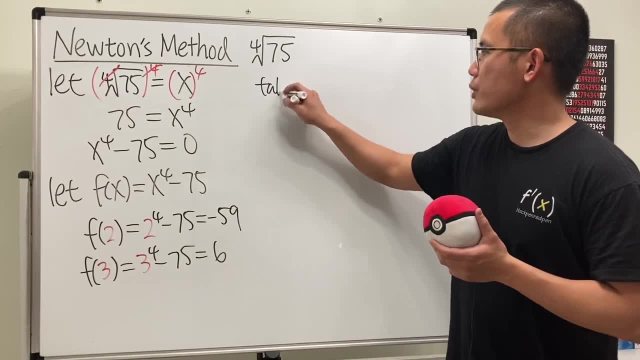 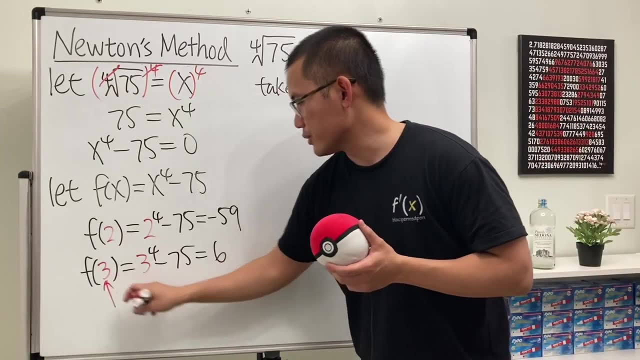 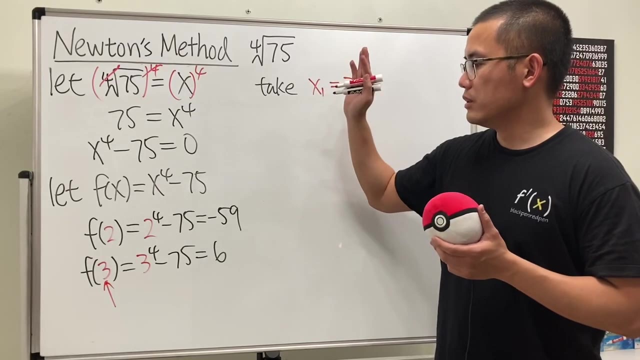 So I'm just going to say We will take And our initial guess, which I will denote, that by x1.. And we will just say: that's equal to 3, right here, This is our initial guess, Again, because the force root of 81 is 3.. 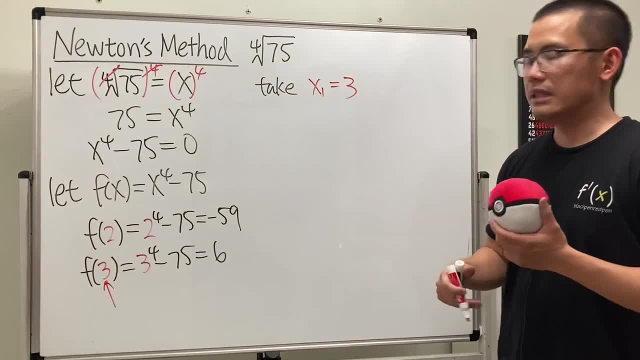 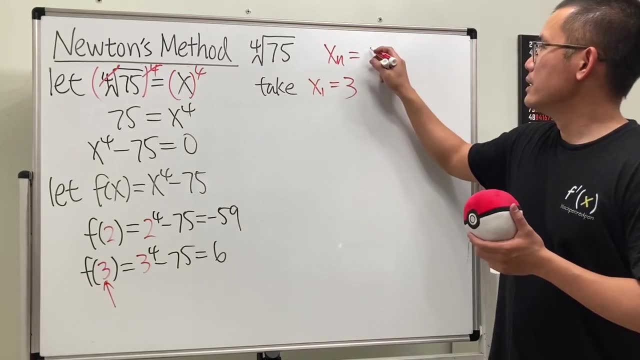 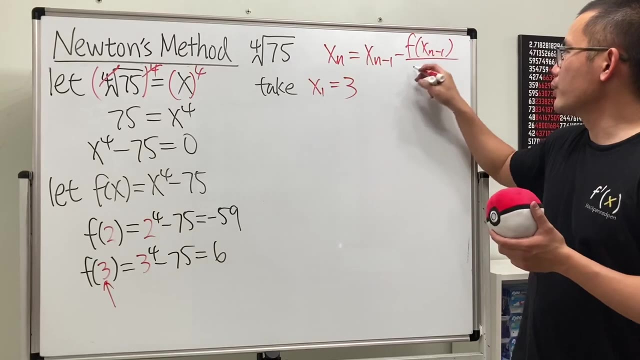 And then we are talking about force root of 75. So this is pretty good And let's just go ahead and get to work. Remember the formula is: xn equals the previous term Minus the previous term for the value of the function. 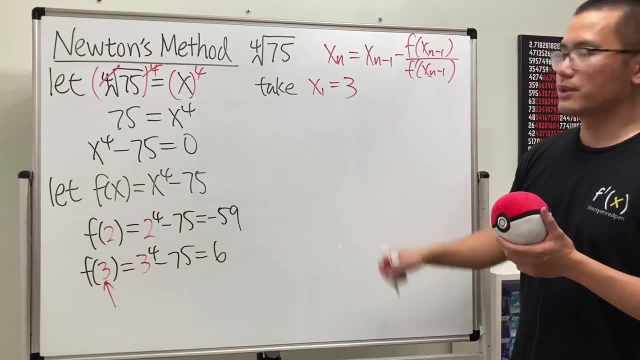 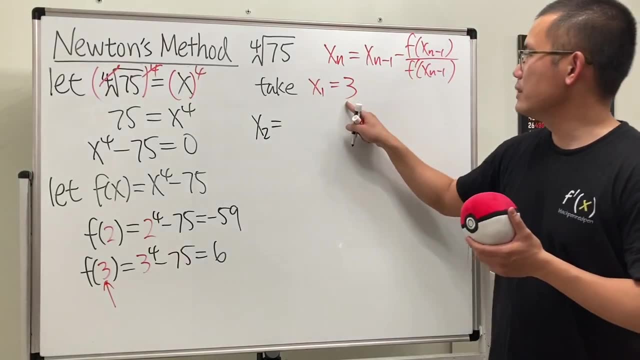 And then the derivative. All right, And then let's just go ahead and get to work, All right. So this is x1.. Now let's see x2.. We will be putting 3 into here And then putting 3 into the function. 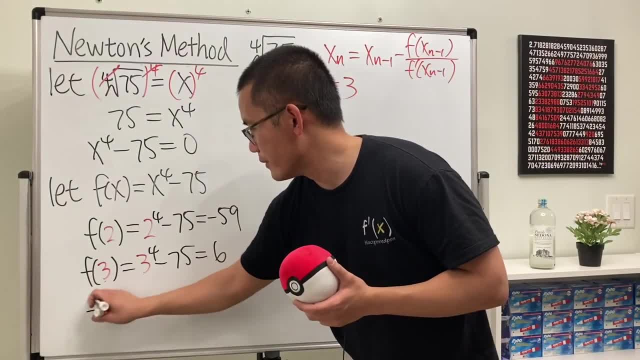 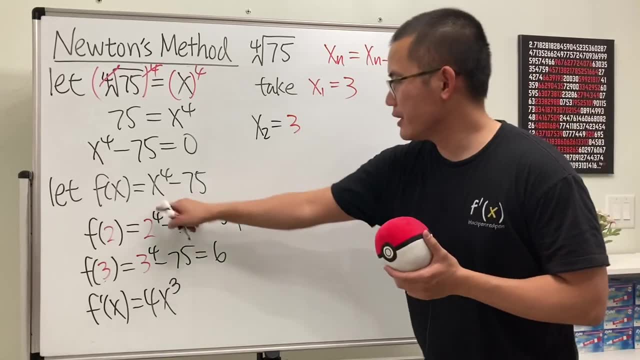 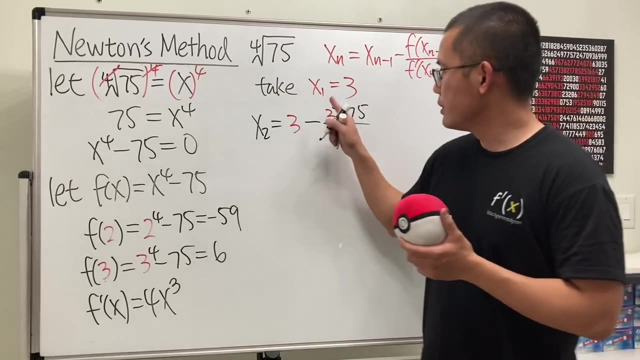 Oh, we also need the derivative, So perhaps I'll put down the derivative right here. Derivative is 4x to the third power, Okay, 3.. Put it here: We get 3 to the fourth power minus 75 over putting 3 into here. 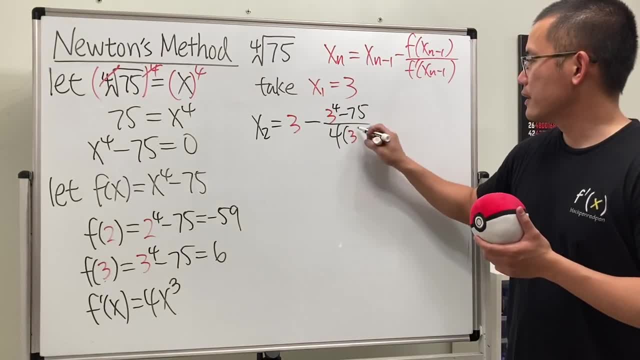 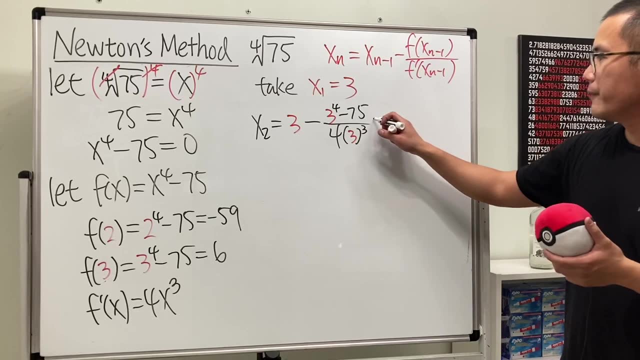 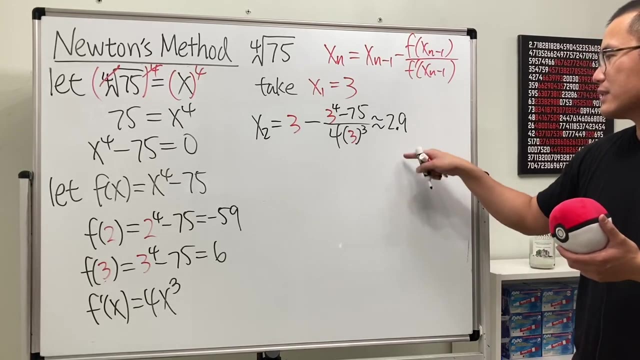 Yeah, So just work that out. Yeah, And then just work that out. I will see This right. here is 2 point, Approximately 2.9.. And then we want a total of 8 digits after the decimal point, So, okay, 9.. 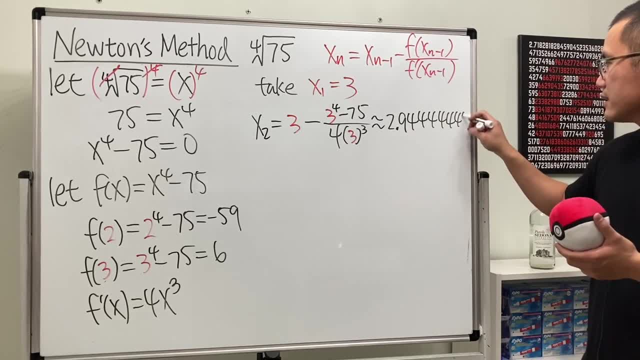 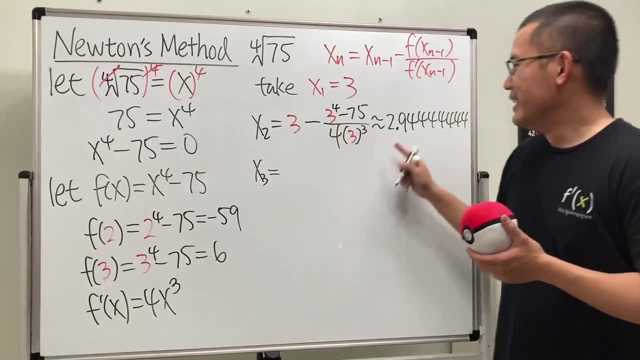 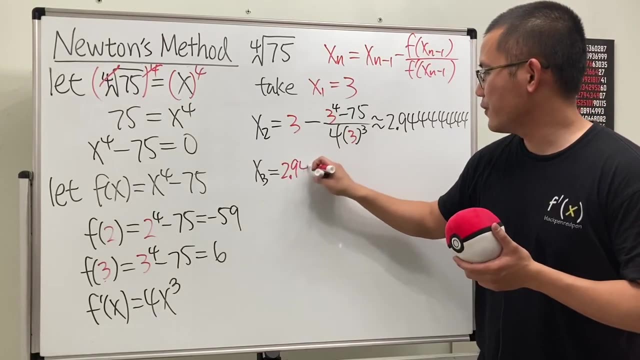 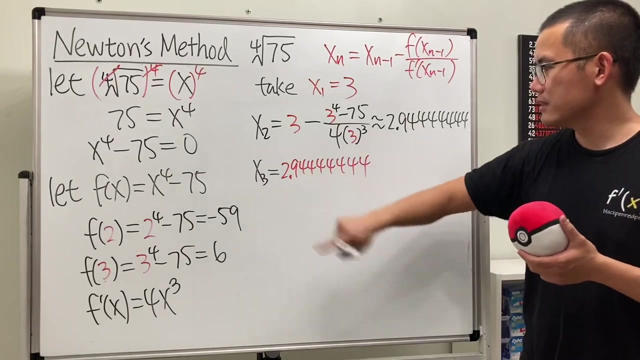 And then 1,, 2,, 3,, 4,, 5,, 6,, 7,, 7, fourths and that. so yeah, okay, x3. Putting this into here and also all the stuff. So yeah, you know the 2.9444444 and 1,, 2,, 3,, 4,, 5,, 6,, 7, so 8 digits minus, put it here. 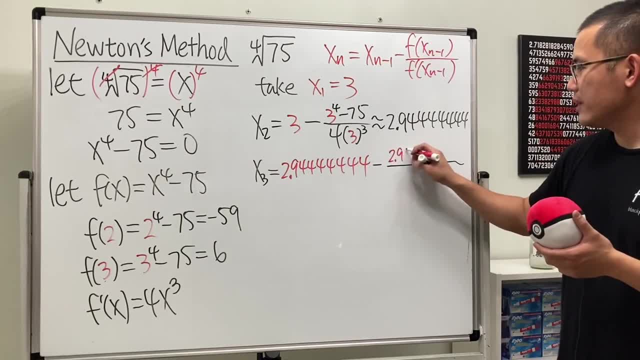 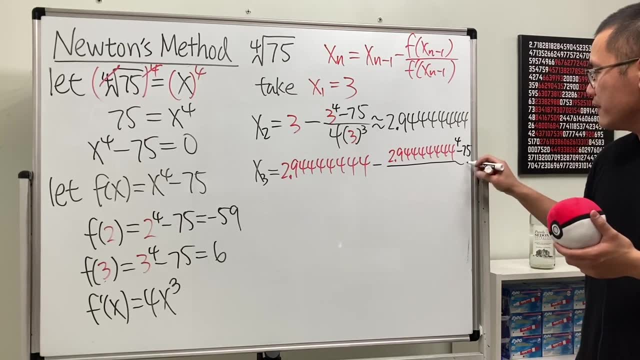 into the function, So 2.9,, 1,, 2,, 3,, 4,, 5,, 6,, 7 to the fourth power, and then minus 75 over 4 times 2.1234567 to the third power. 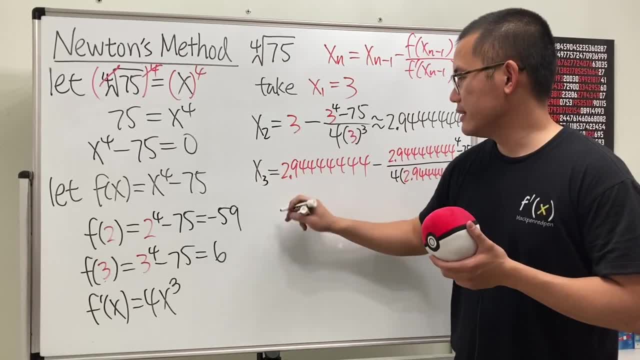 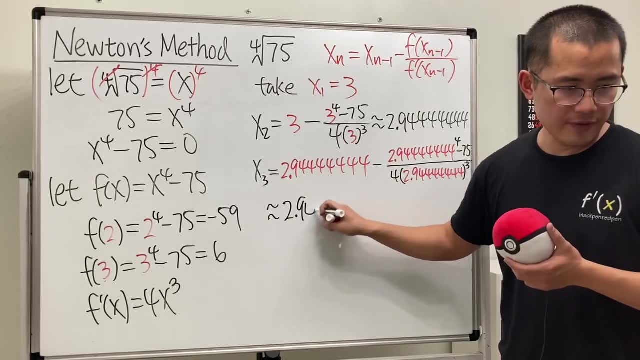 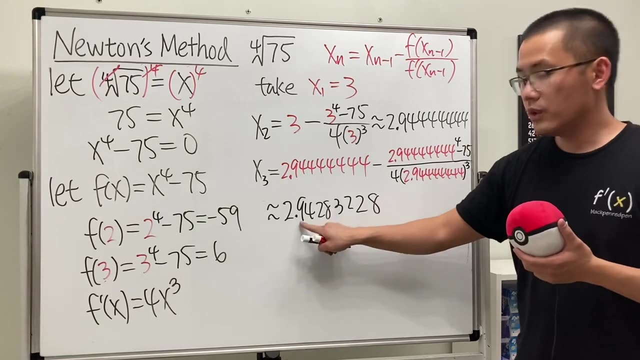 Yeah, And just keep doing it. That's all. And this right here will be appropriate. Okay, Approximately okay: 2.9428322NN28.. So we do see that we have 8 digits, right, 8 decimal places, but this and that are not. 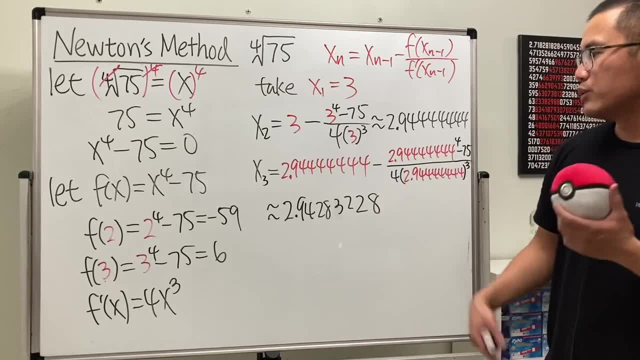 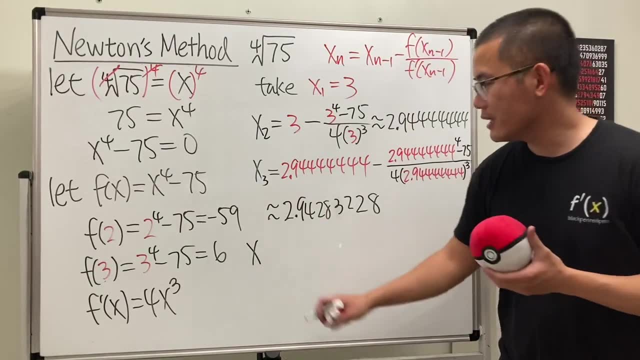 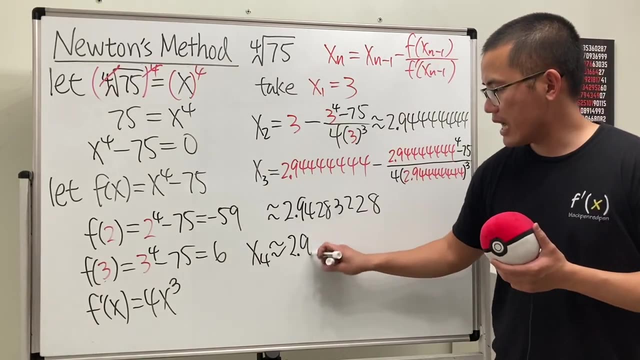 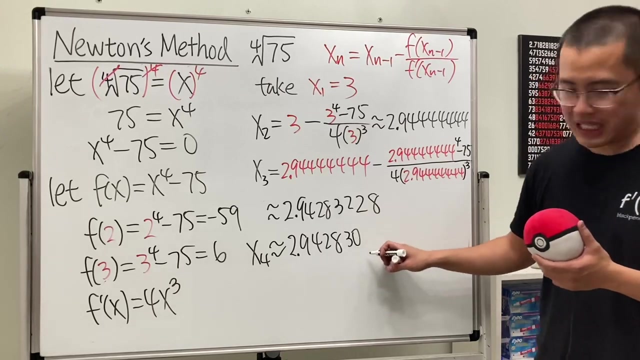 the same. Yes, So we'll just have to run through the iteration again, but it's the same thing. So I'm just going to write down the next iteration. if you were going to plug in everything, X4 will be approximately. we get 2.9428 and then 30956, about to run up, so it'll be 96. 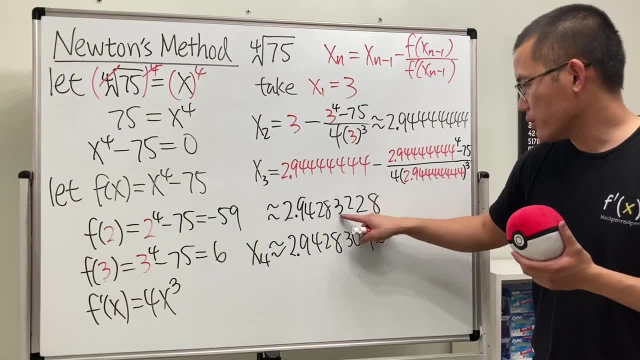 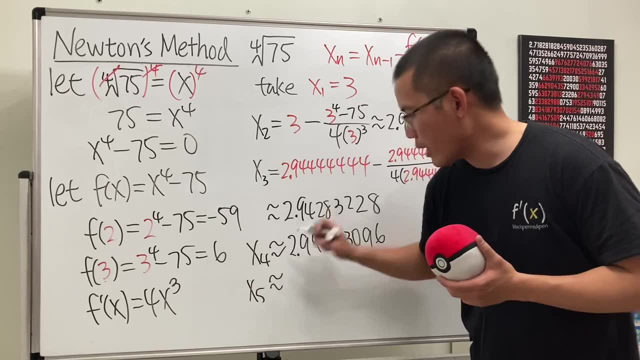 right here And you can see that, oh, it's off by right here, right? So let's see If we do this again. X5, it will be approximately 2.9428322NN28.. Okay, Okay. 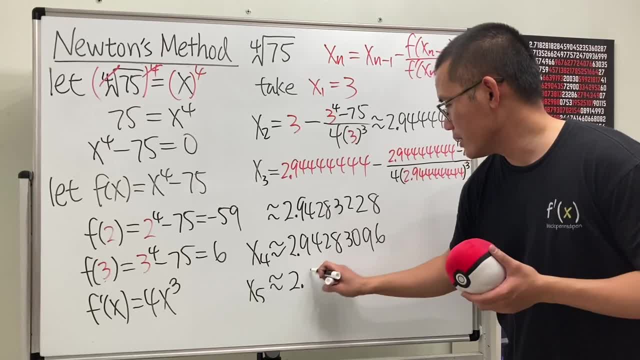 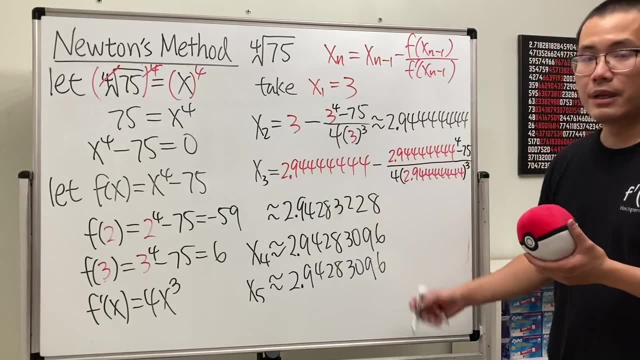 So this is actually in fact, almost identical. Yeah, And the first 8 digits after decimal point it's actually. they are actually the same, So we can see that we don't have to continue because, yeah, this is pretty much it, because 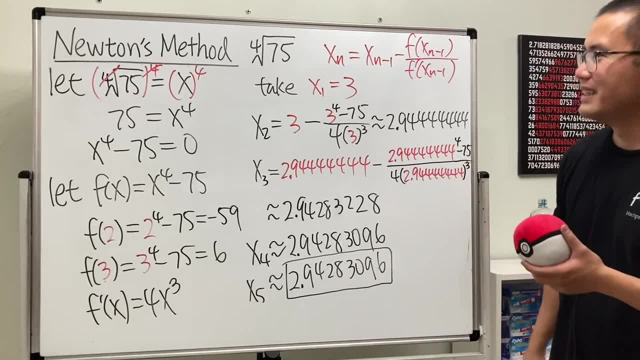 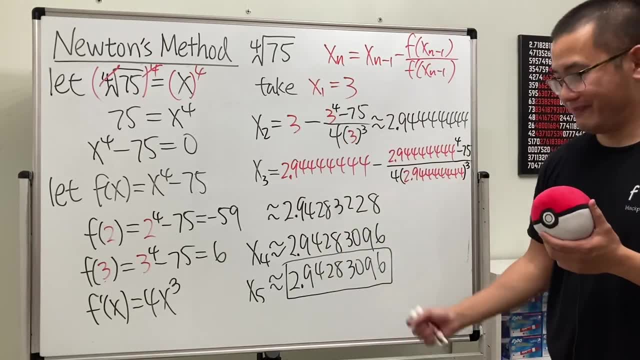 the more you do it. yeah, you cannot see the changes after that. So this will be a super good approximation for this. after just like two or three iterations, That's it.